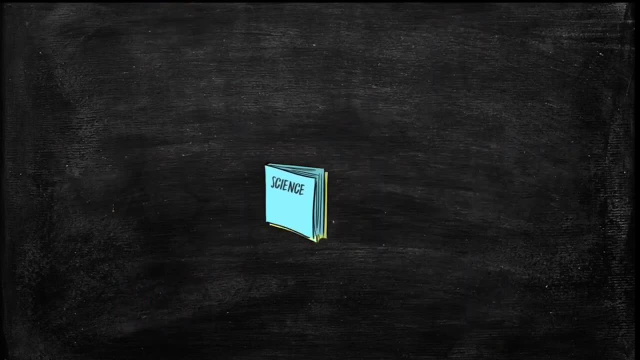 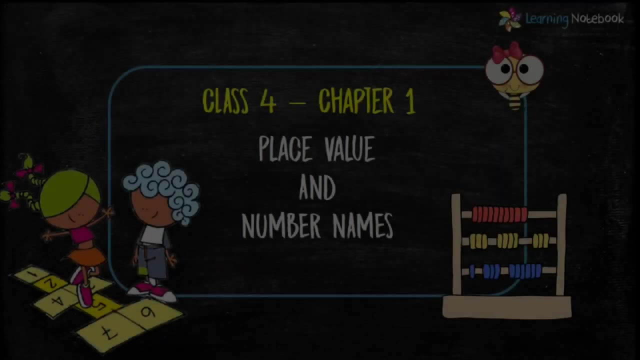 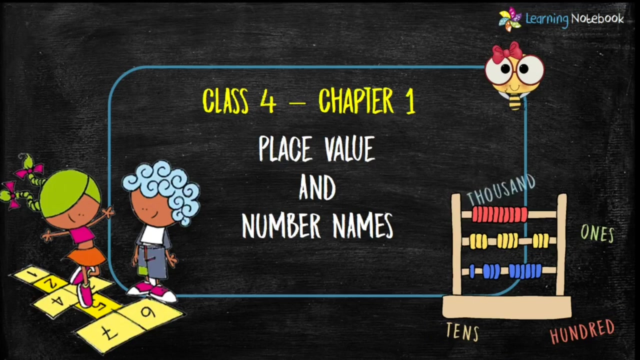 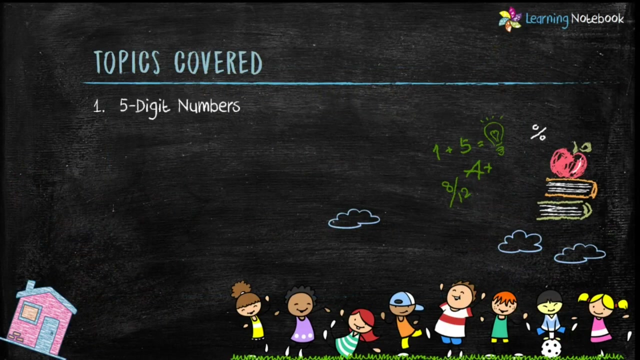 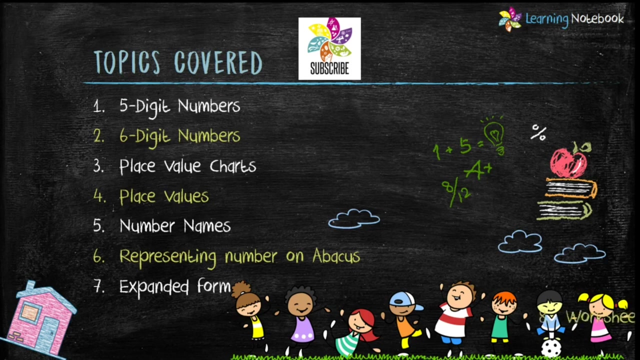 Welcome students to class 4, chapter 1: place value and number names. Today we are going to cover the following topics under this chapter: 5: digit numbers. 6 digit numbers. place value charts. place values, number names representing number on abacus, expanded form and in the 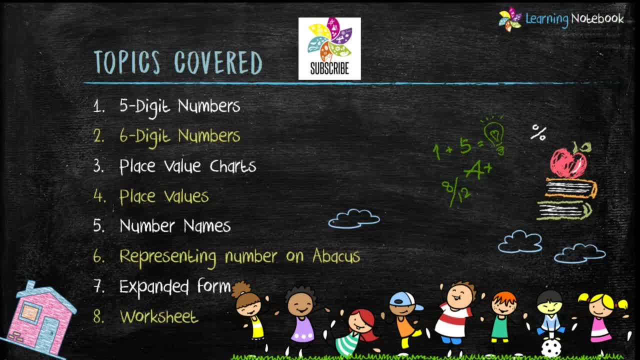 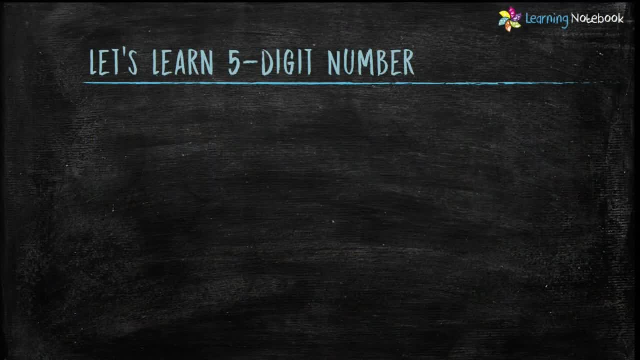 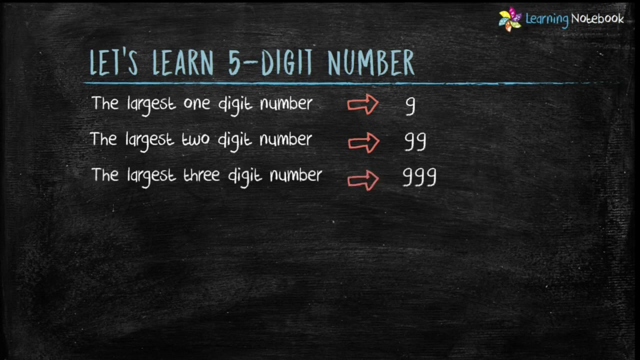 last, I will provide you a worksheet to practice upon. Let's learn 5 digit numbers. As we already know, the largest 1 digit number is 9.. The largest 2 digit number is 99.. The largest 3 digit number is 999.. The largest 4 digit number is 9999.. So what is 9999 plus 1?? It is 10000, or we call it. 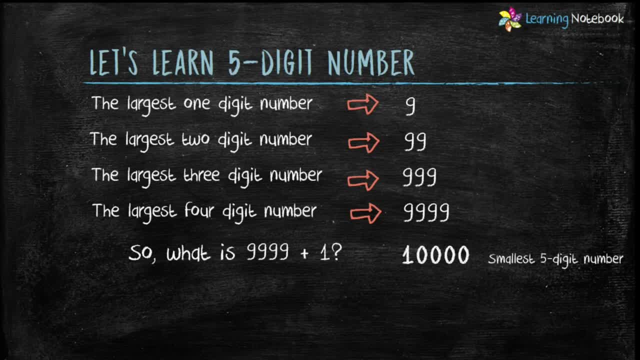 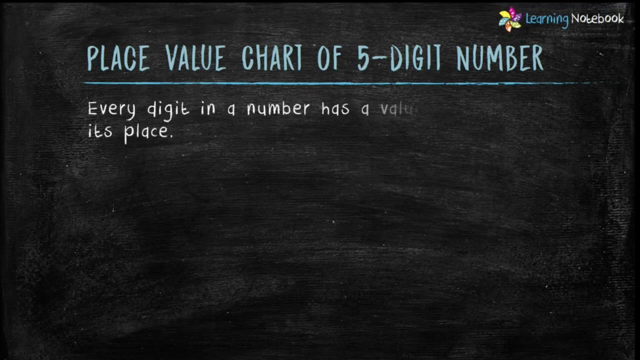 5000.. This is the smallest 5 digit number. Now what is the largest 5 digit number? 99999.. We will learn about how to name 5 digit number in a short while. Now let's understand place value. chart of 5 digit number. What is place value? Every digit in a number has a value. 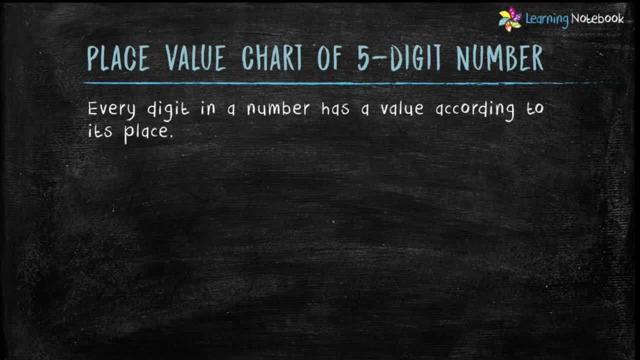 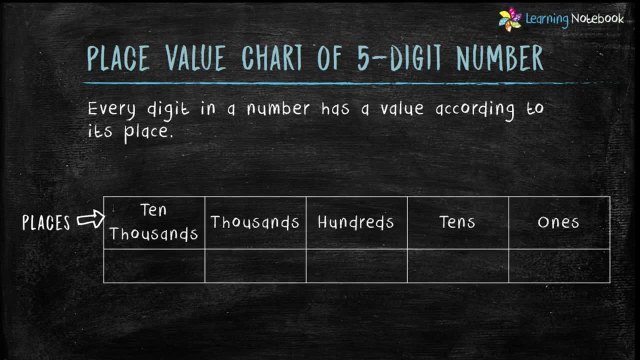 According to its place. This is called as Place value. So let's see what all places we have in a 5 digit number, Starting from left, we have 1s, 10s, 100s, 1000s and then 10000s. 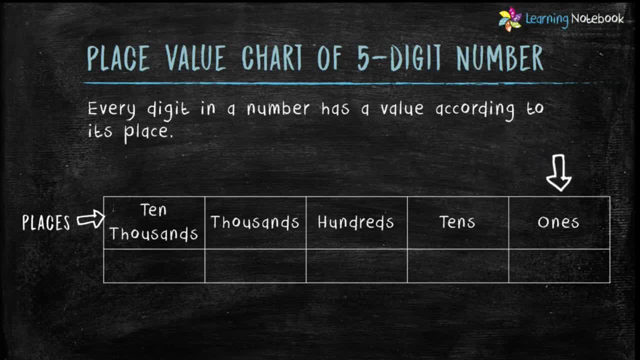 Where 1s is denoted by O, 10s is denoted by T, 100s is denoted by U and 1000 has the same value as 0. So what is place value? The base value is the number 10.. So the base value of almost every digit is a 5 digit number in the number 1 and 10.. Now let's see what all places are in a 5 digit number. Starting from left. we have ones 10s, 100s, 1000s and then 10000s. 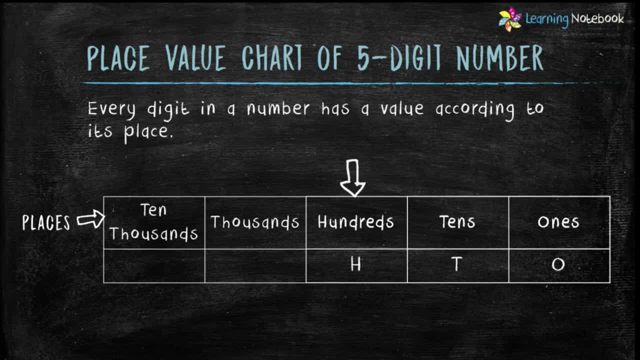 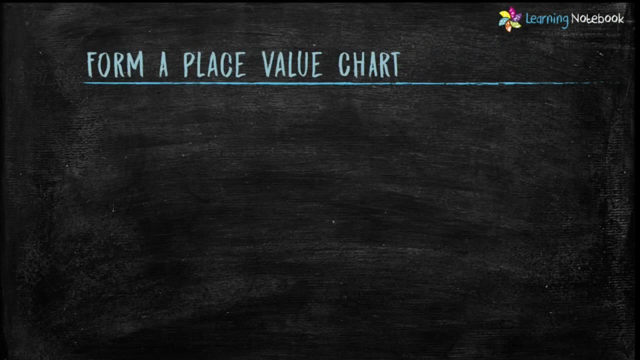 100s is denoted by H, 1000s is denoted by TH and 10000s is denoted by TTH. Now, students, let's form a place value chart for a 5 digit number with the help of an example. 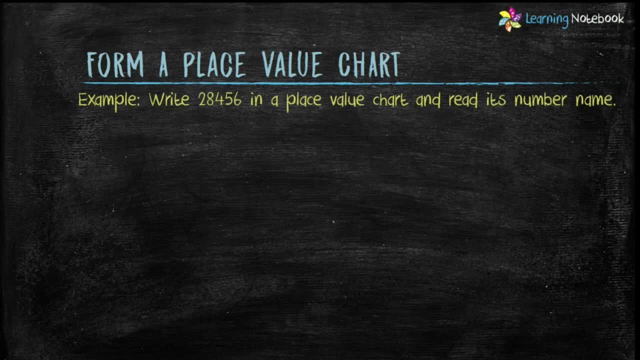 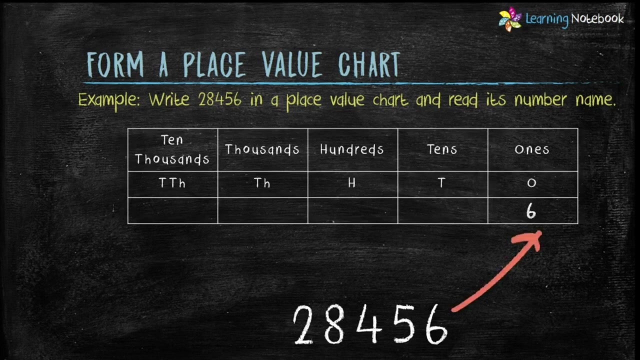 Example is to write 28456 in a place value chart and read its number name Here starting from left. since 6 is at 1's place, let's put 6 in the 1's place in the place value chart Now. 5 is at 10's place, 4 is at 100's place, 8 is at 1000's place. 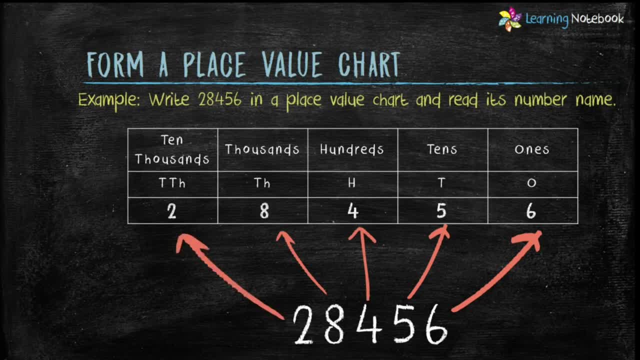 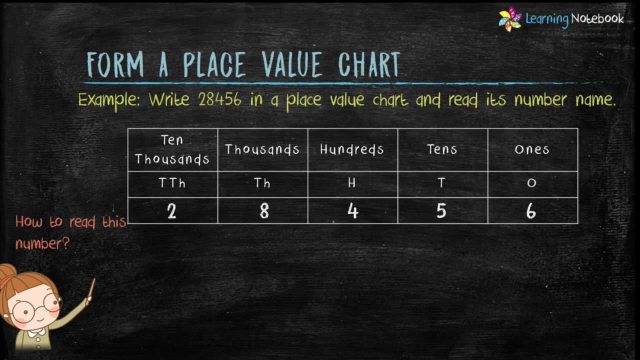 And 2 is at 10,000's place. So this is how we make a place value chart for a 5 digit number. Now I will tell you how to read this number or its number name. Students always first read 1000's places together. 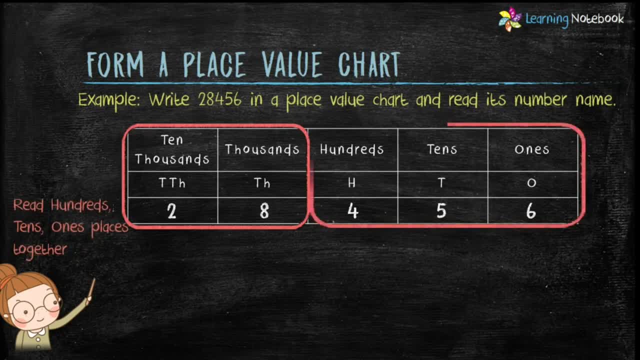 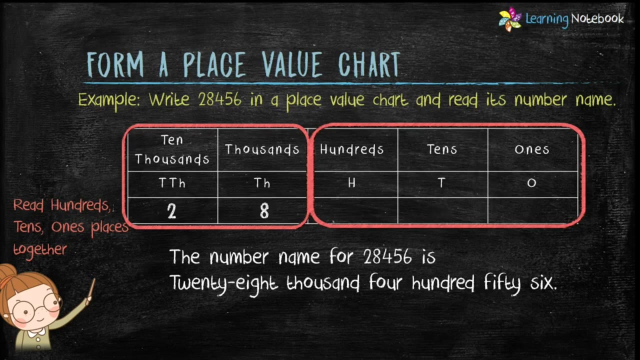 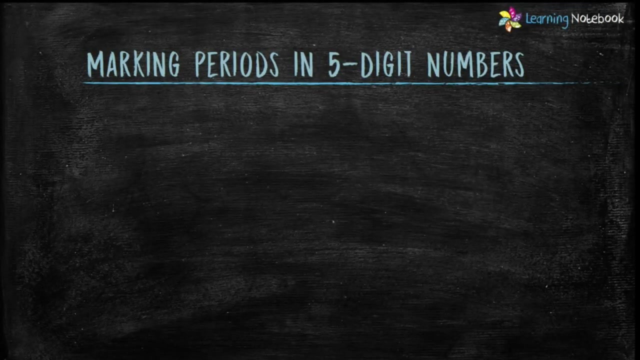 Then read 100's, 100's, 10's, 1's places together. So the number name for 28456 is 28456.. Students, let's learn how to mark periods in 5 digit numbers. It is very simple to mark periods on the number. 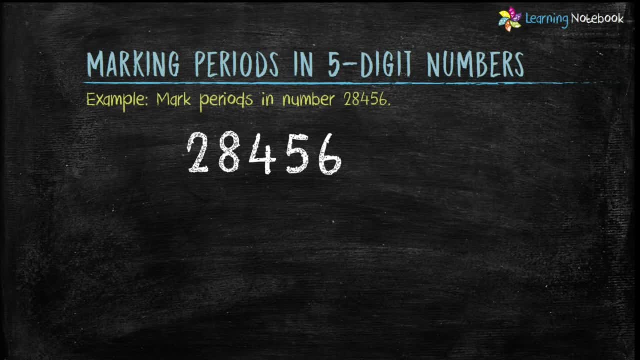 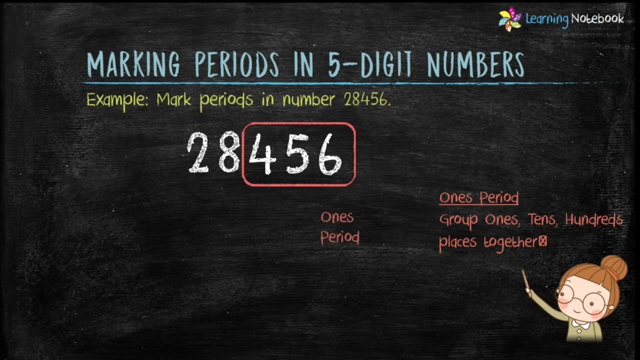 And it is used to Easily read the big numbers. Here we have an example to mark periods in number 28456.. So first period is 1's period, which is the group of 1's, 10's and 100's places. 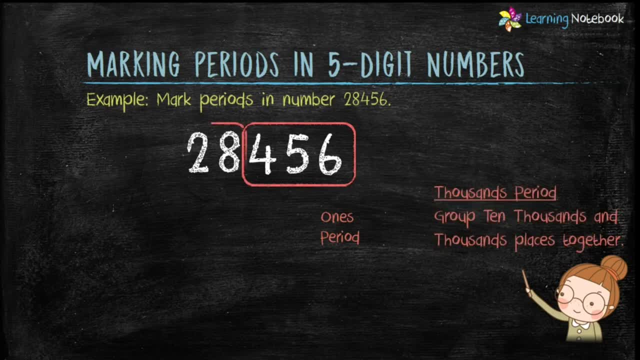 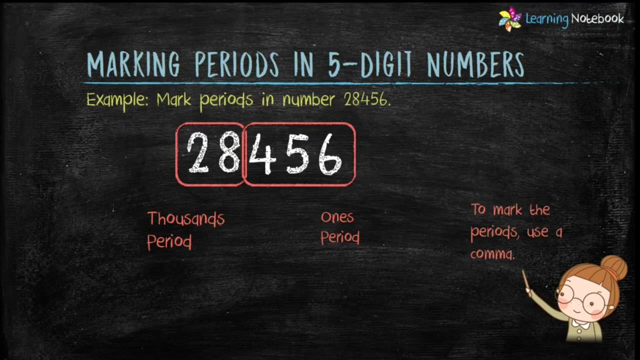 Second period is 1000's period, which is the group of 1000's and 10,000's places. To mark the periods we use a comma in between 1's and 1000's period. So in this example- 28456,, we will use a comma between 1000's period and 1's period. 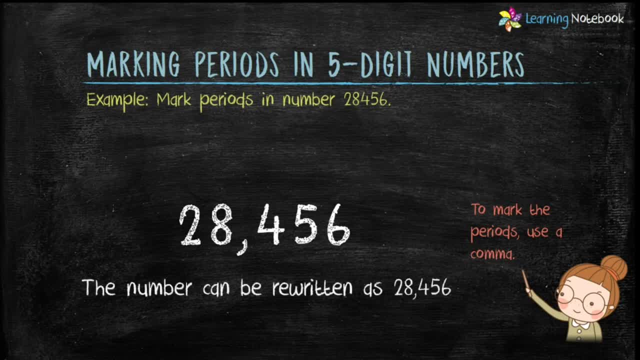 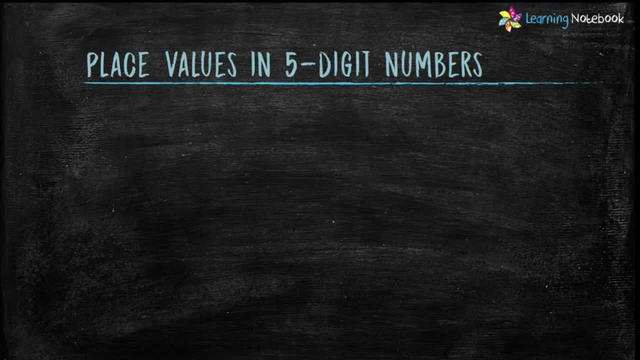 Thus this number can be rewritten as 28456.. Students, now let's learn how to write this number: place values in five-digit numbers. Example is to write the place values of each digit in 79536 and write its expanded form. Let's quickly make a place value chart, as we did before. 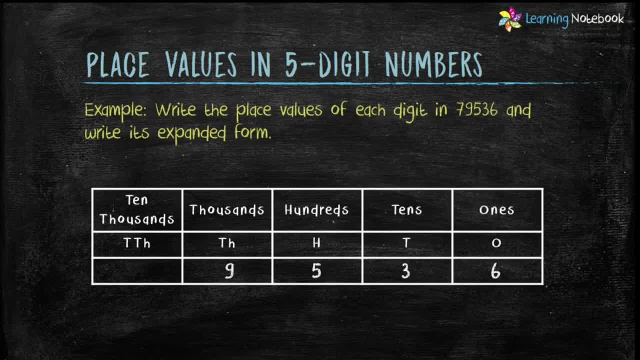 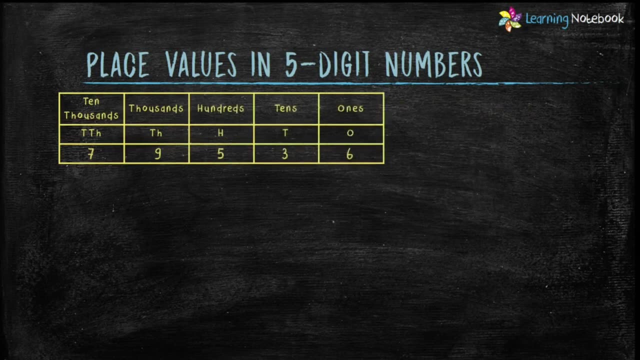 Now let's put 6 at 1's place, 3 at 10's place, 5 at 100's, 9 at 1000's and 7 at 10,000's place. Let me make this table a little bit smaller. Now here, since 6 is at 1's place, its place value is: 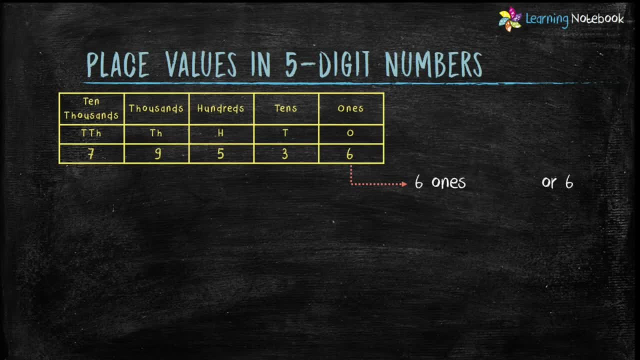 6, 1's or 6.. Then 3 is at 10's place, so its place value is 3, 10's or 30.. 5 is at 100's place, so its place value is 500's or 500.. 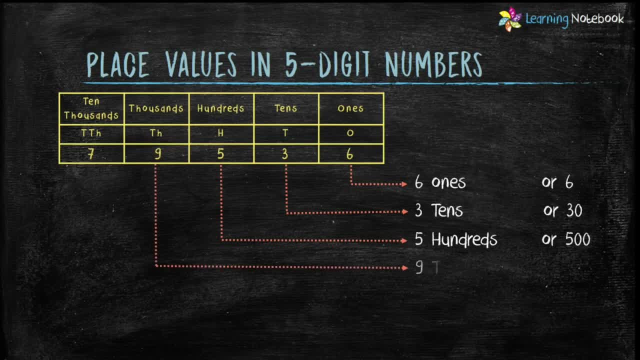 9 is at 1000's place, so its place value is 9000's or 9000.. And lastly, digit 7 is at 10,000's place, so its place value is 7, 10,000's or 70,000's. 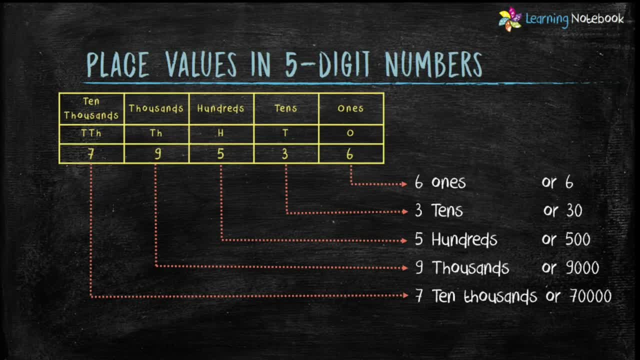 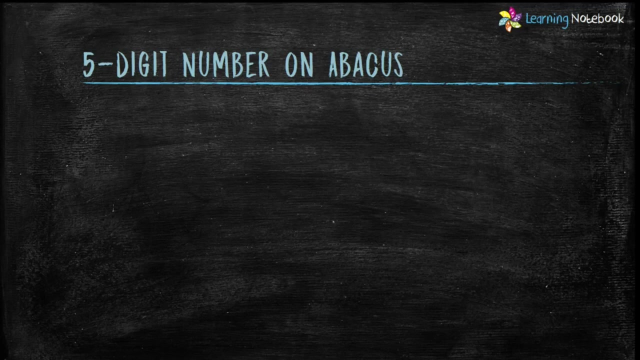 Now we can easily write the expanded form of this number, which is 70,000 plus 9,000 plus 500 plus 30 plus 6.. So, student, this is how we will write the place values of 5 digit numbers and their expanded form. Now let's see how to represent 5 digit number on abacus. 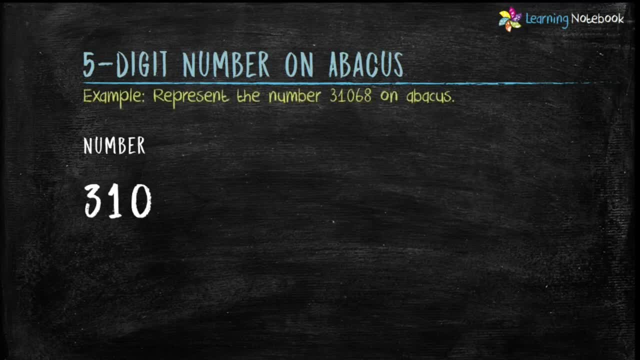 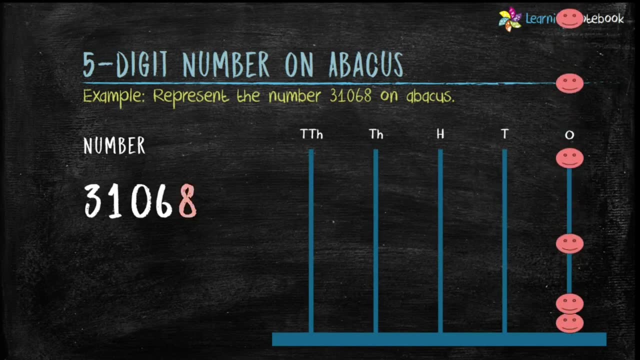 Example is to represent the number 31068 on abacus. Since we have 8, at 1's place, we will put 8 beads at 1's spike. Next we have 6 at 10's place, so put 6 beads at. 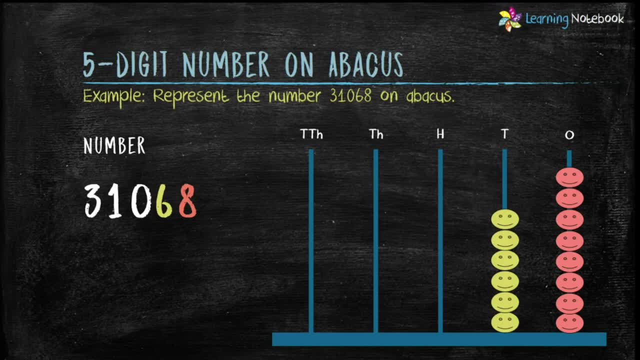 10's, Then 0 at 100's place, so i will not put any if 4 at 100,, who means 7 Fs. Next we have 1 at 1000's place, so let's put 1 bead at 1000's spike. 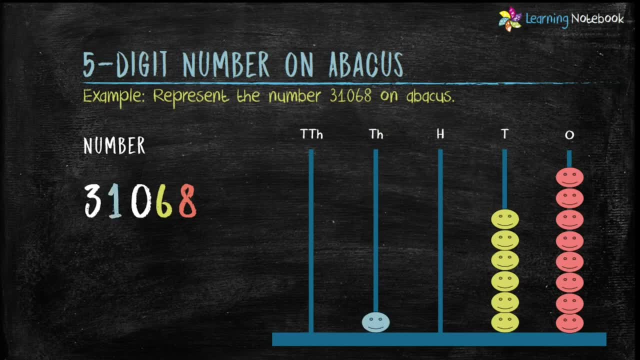 So let's done. And lastly, we have 3 at 10,000th place, So we will put 3 beads at 10,000th spike. So, students, this is how we represent 5 digit number on a backers. 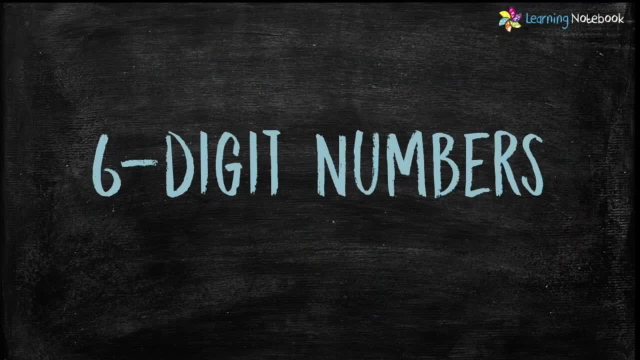 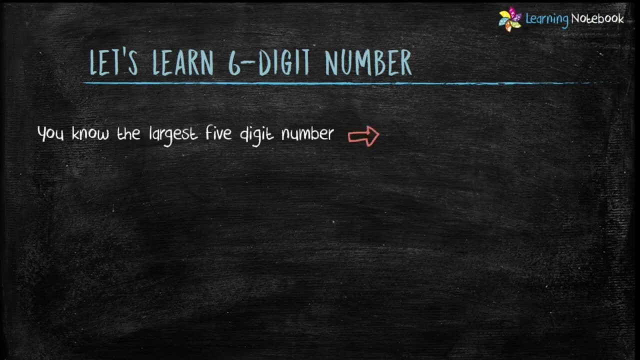 Students, we have now learnt 5 digit numbers. Let's proceed to learn 6 digit numbers. We already know that the largest 5 digit number is 99,999.. So the question is: what is 99,999 plus 1?? 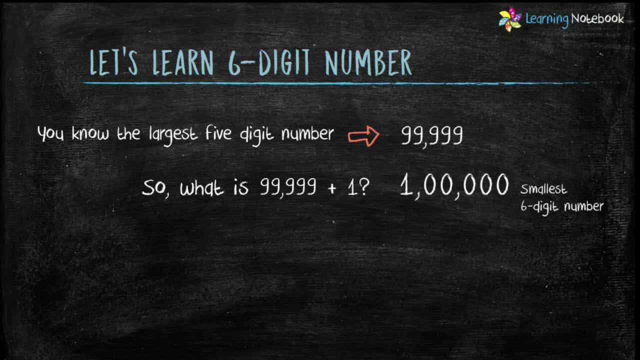 It is 100000, or we call it 1 lakh. This is the smallest 6 digit number. Now, what is the largest 5 digit number? What is the largest 6 digit number? It is 999999, or we can read it: 9,99,999.. 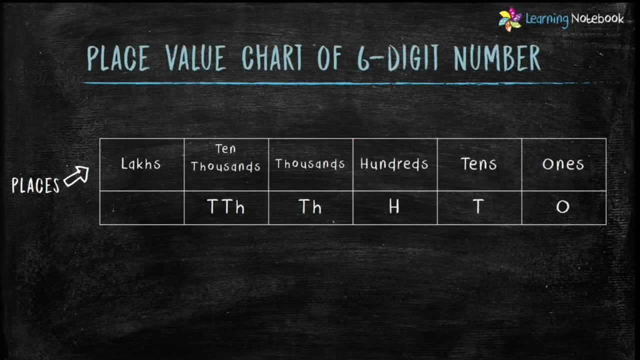 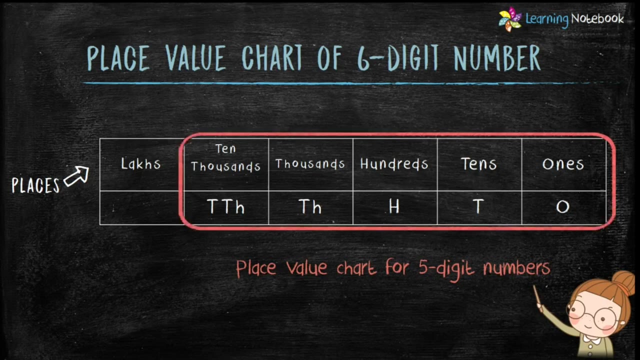 Now, students, let's understand place value chart of 6 digit number. We just learnt place value chart for 5 digit numbers, So we have 1s, 10s, 100s, 1000 and 10,000.. 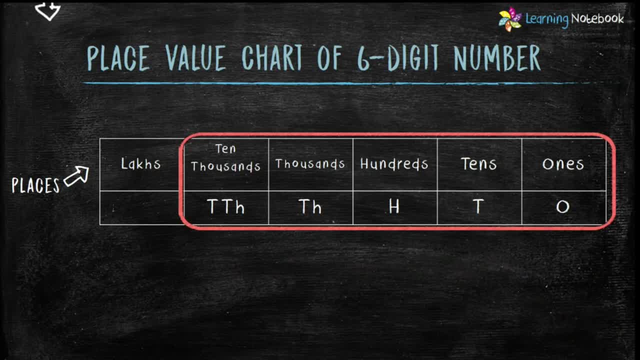 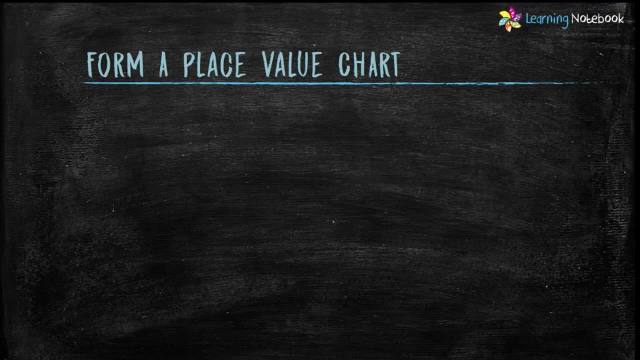 We have 6th place in 6 digit number. It is known as lakhs and is denoted by L Students. let's form a place value chart with the help of an example. Example is to write 9,, 2,, 8,, 4,, 5,, 6 in a place value chart and read it's number name. 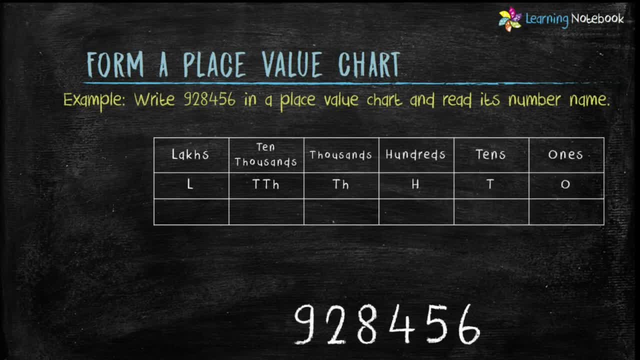 Here, starting from left. since 6 is at 1's place, let's put 6 at 1's place in place. value chart Now: 5 at 10's place, 4 at 100's place, 8 at 1000's place. 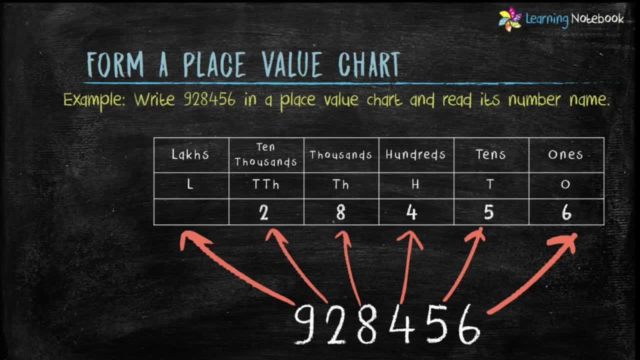 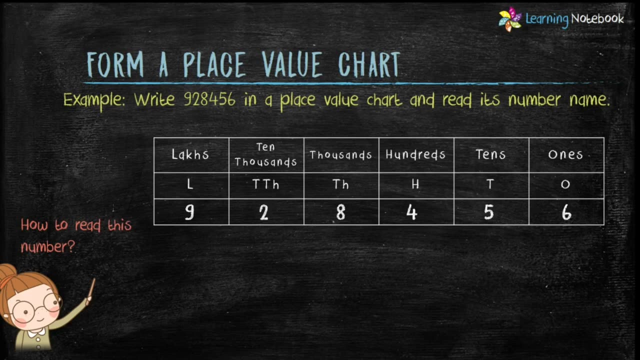 2 at 10,000's place And, lastly, 9 at lakh's place. This is how we make a place value chart for 6 digit number. Now I will tell you how to read this number or how to write its number name. 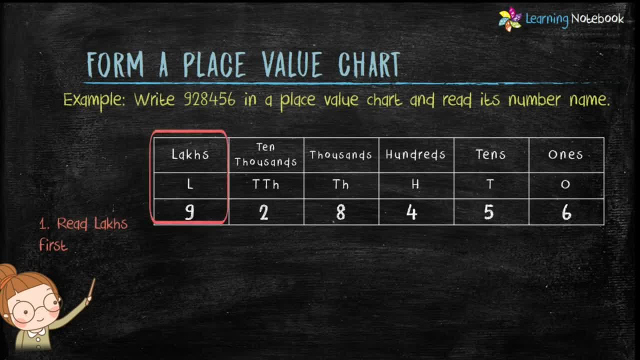 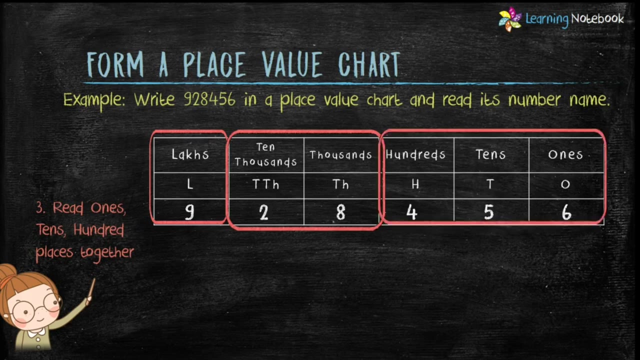 First read lakhs, Then read 1000's places together And lastly read 1's 10's 100's places together. So the number name for 9,, 2, 8,, 4, 5, 6 is 9, 28, 456.. 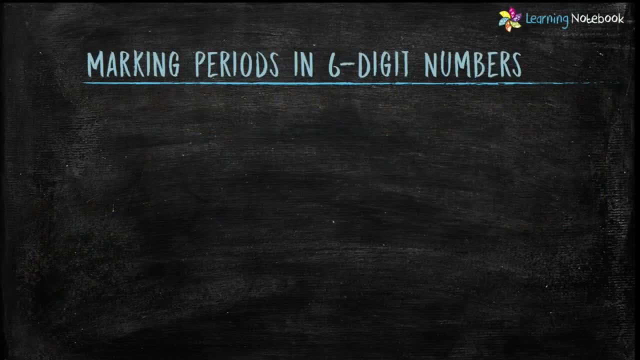 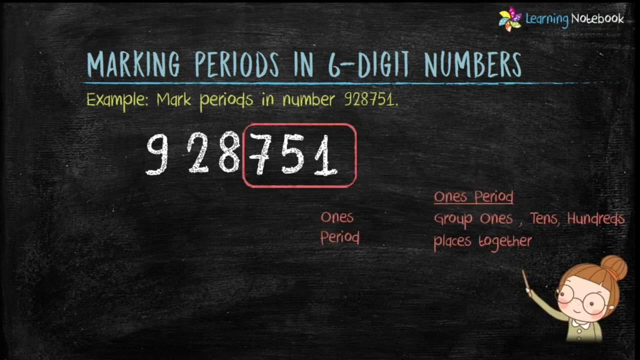 Students, let's learn how to mark periods in 6 digits. It is very simple to mark periods on the number and is used to easily read the big numbers. First period is 1's period, which is the group of 1's, 10's and 100's places together. 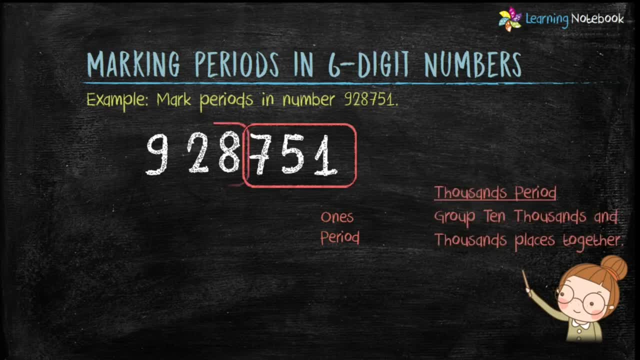 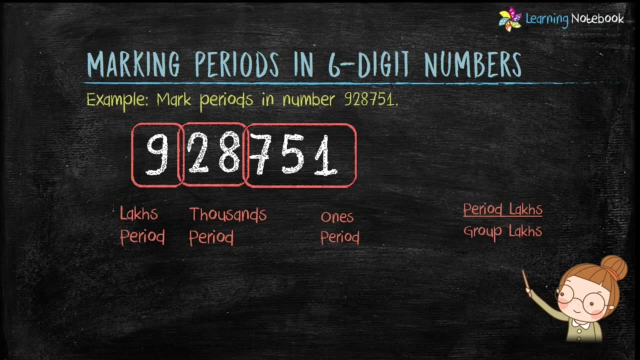 Second period is 1000's period, which is the group of 1000's and 10,000's places together. And third period is the lakh's period. This is the period of lakhs. So to mark the periods we use comma in between 1's period, 1000's period and lakh's period. 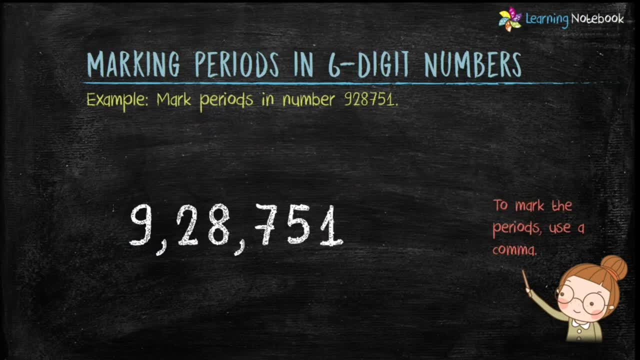 So in this example, 9,, 2,, 8,, 7,, 5, 1.. We first put a comma in between 1's and 1000's period and then another comma between 1000's and lakh's period. 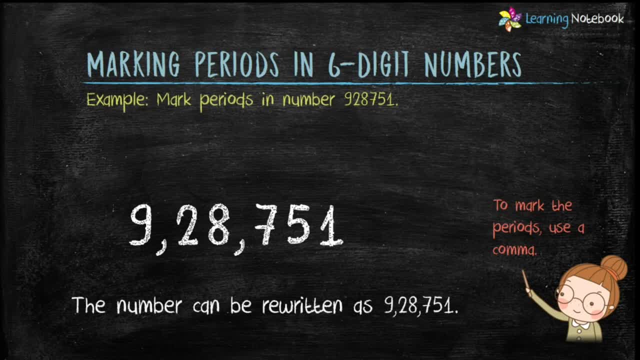 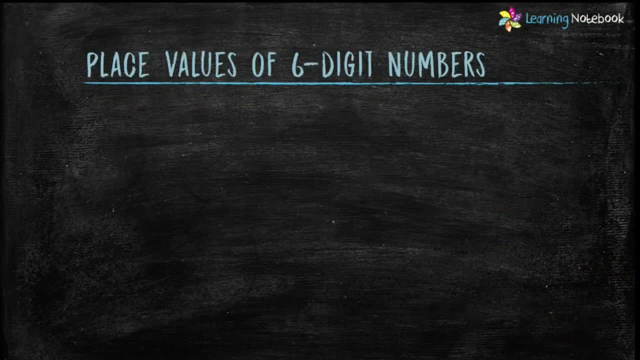 So this number can be used can be rewritten as 9,28,751. Students. now let's learn the place values of 6 digit numbers with the help of an example. Write the place values of each digit in 879536 and write its expanded form. First, let's quickly make a place value chart. 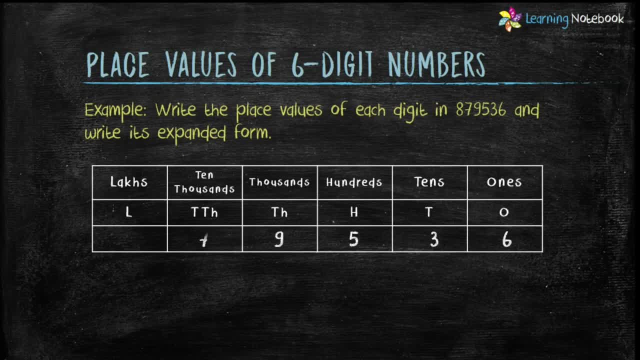 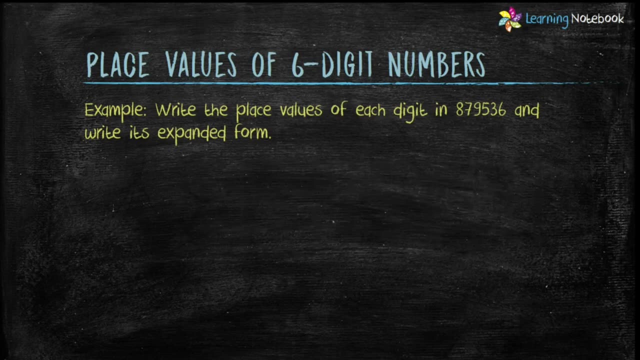 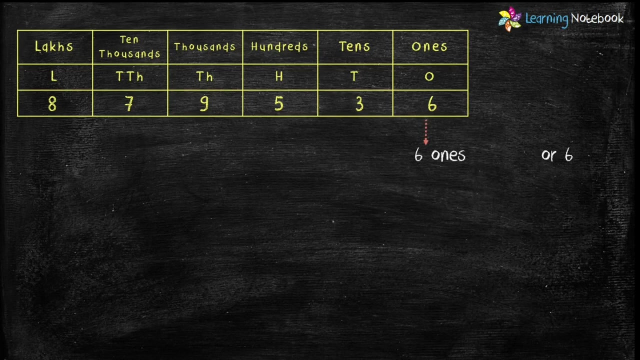 as we did before, Let me make this table a little bit smaller Now. since 6 is at ones place, its place value is six ones or six. Now. 3 is at tenths place, so it is less than the second and the third digit number plus 7 times ten is even more than the middle digit number. 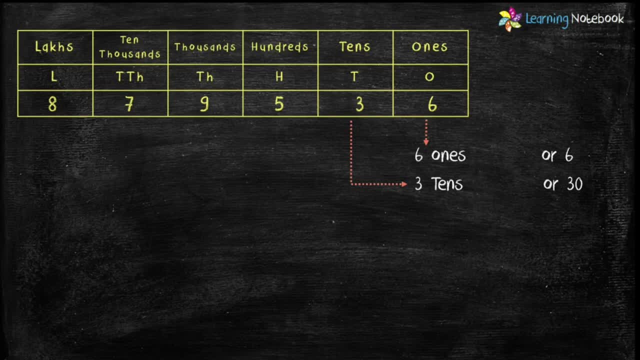 So it's less than the first digit and more than the third digit number. its place value is 3 tens or 30.. Similarly, 5 is at 100's place, So its place value is 500's or 500.. Now, 9 is at 1000's place, So its place value is 9000's or 9000.. Next, 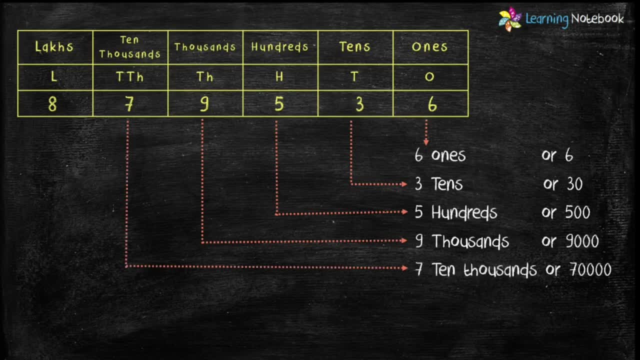 we have 7 at 10,000's place, So its place value is 7, 10,000's or 70,000.. And lastly, we have 8 at lakh's place, So its place value is 8 lakh's or 8 lakh Students. now we have 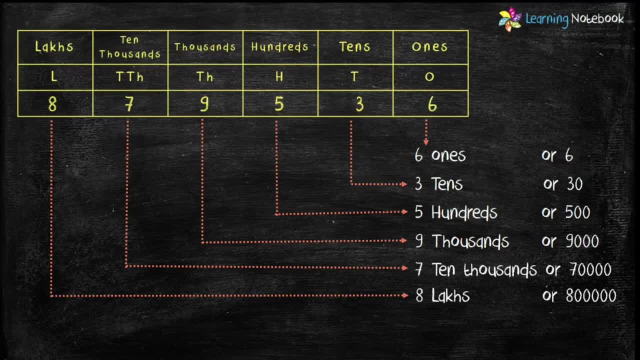 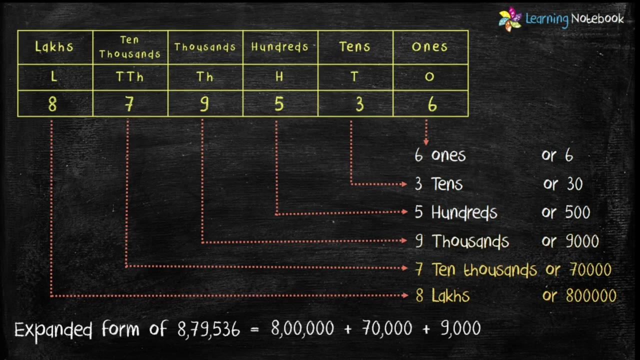 these place values. So let's see how to write the expanded form of a 6-digit number. Expanded form of 8, 7, 9, 5, 3, 6 equals to 8 lakh plus 70,000 plus 9000, plus 500, plus 30 plus 6.. Now it is time. 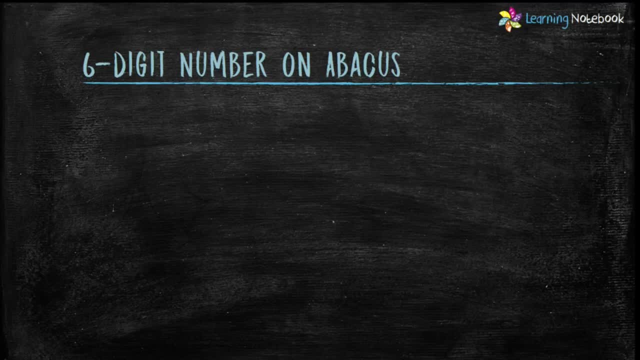 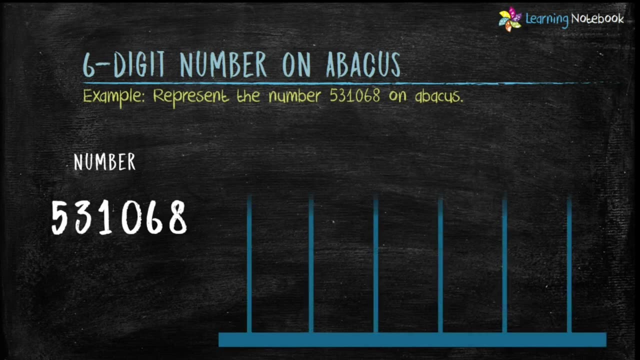 to learn how to represent 6-digit number on a backers. Example is to represent the number 5, 3, 1, 0, 6, 8.. Since we have 8 at 1's place, we will put 8 beads at 1's spike. Next we have 6 at 10's. 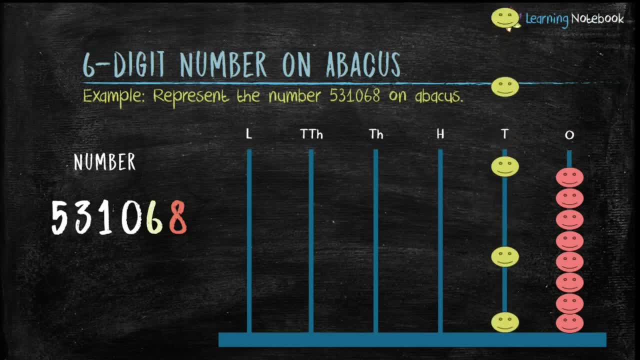 place. So put 6 beads at 10's spike, Next 0 at 100's place, So we will not put any beads at 100's spike. Then we have 1 at 1000's place. So let's put 1 bead at 1000's spike.